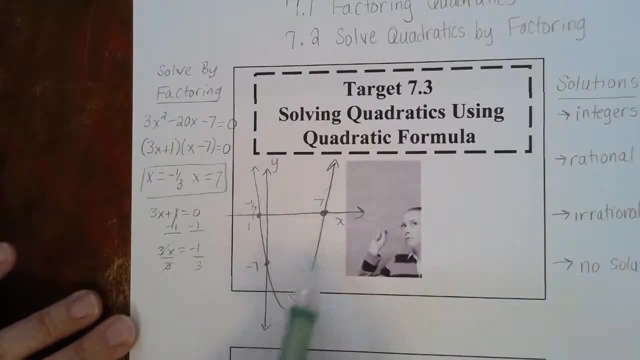 You could also graph, which we'll get into in, I believe, Target 7.4 to find the solutions. The solutions are where it crosses the x-axis or the x-intercepts. They're also called roots. 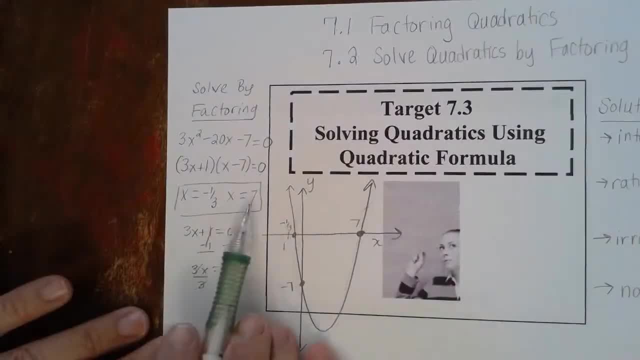 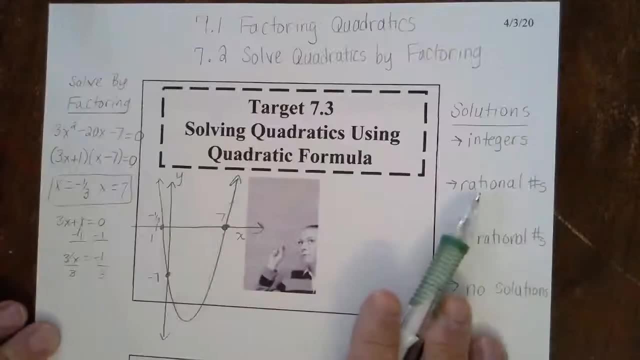 Now our solutions that we had when we factored, we had integers and we had rational numbers, but an integer is a rational number as well. So we could also have fractions for answers when we factored. When we do quadratic formula, we might also get irrational. 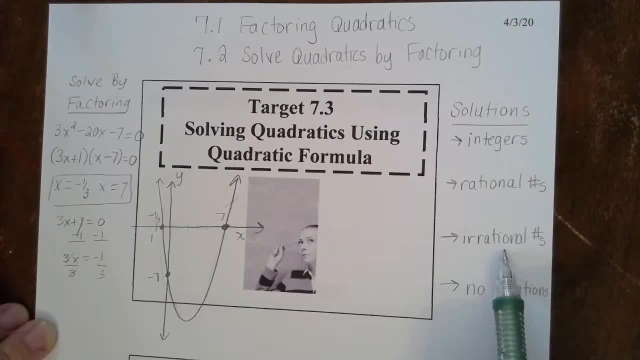 numbers, which are non-repeating, non-terminating decimal numbers. So an irrational number would be something like the square root of 2, or the number pi is also irrational. We may also 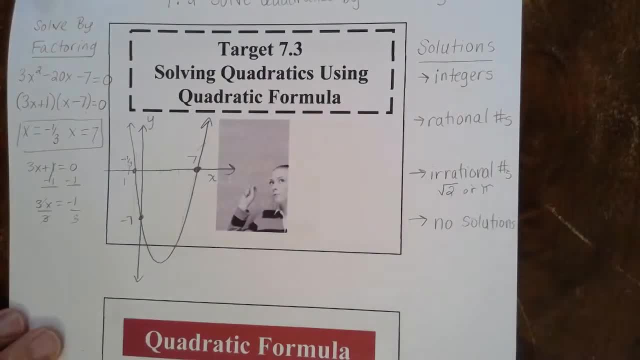 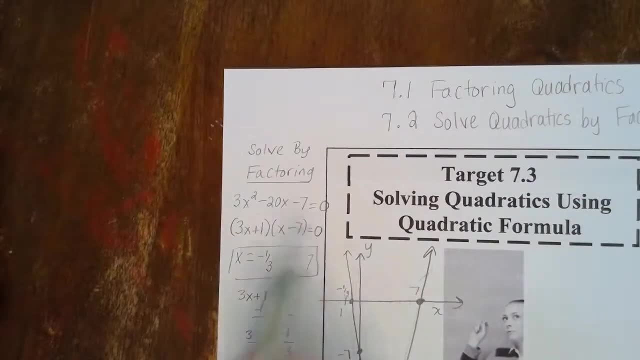 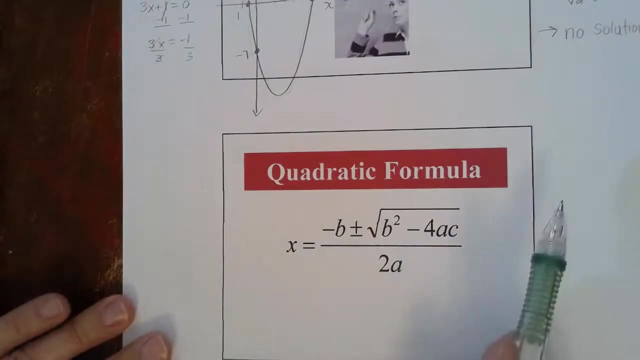 see today a no solution. So you get an error when you apply your quadratic formula. So notice how I said that this is a quadratic equation. Then quadratic formula is a formula kind of just like in geometry. You plug in numbers to get a value at the end. Quadratic formula is a very important formula in algebra because it can solve any quadratic equation. 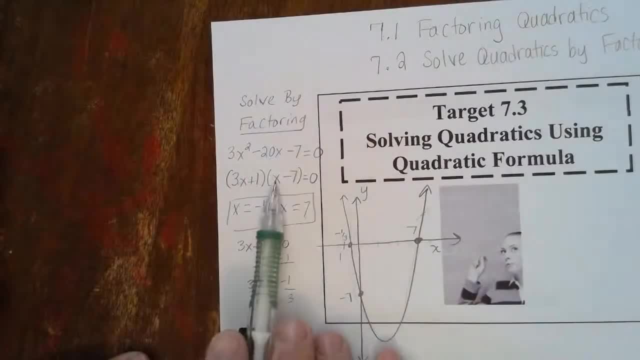 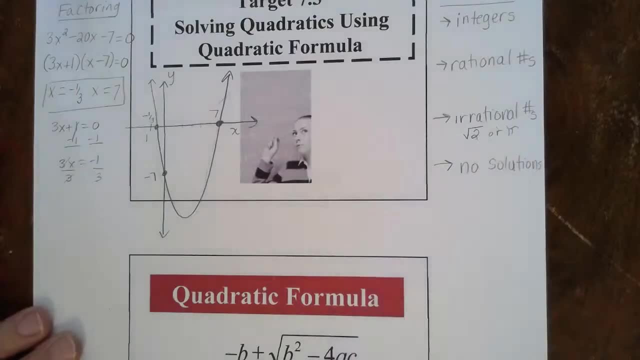 Sometimes equations are not factorable, like this. This is factorable. So you would get maybe an irrational answer for your solutions. So quadratic formula can be used on any quadratic equation. I'm going to go ahead. 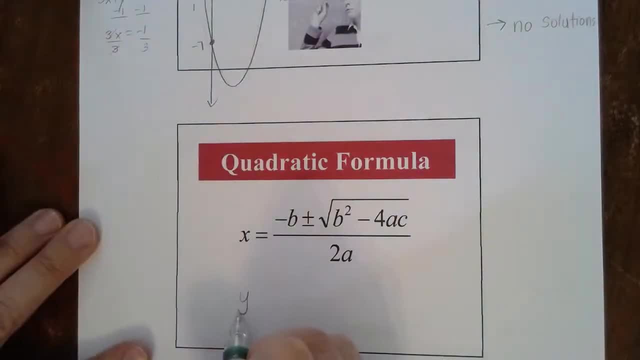 And I'm going to write the equation I had up there, but I'm going to write it as a function. So if I write y equals 3x squared minus 20x minus 7, I have parameters a, b, and c in terms of standard form of a quadratic equation, just like when you have slope intercept or point slope. So you have slope for linear equations. They're these generic forms. Standard form for a quadratic equation is ax squared plus bx plus c. So hopefully you can see that the a value in this quadratic equation is 3. The b value in this quadratic equation is negative 20. 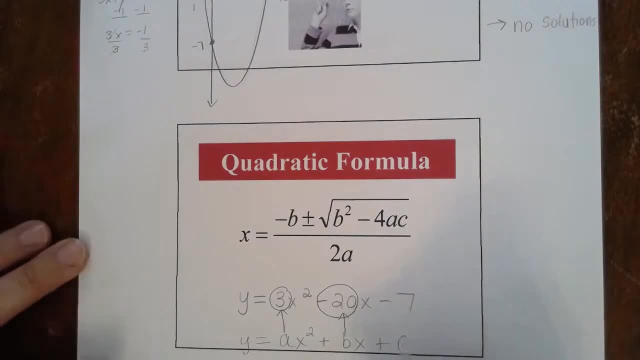 Always take the sign that's in front of the coefficient. And then the c value is negative 7. 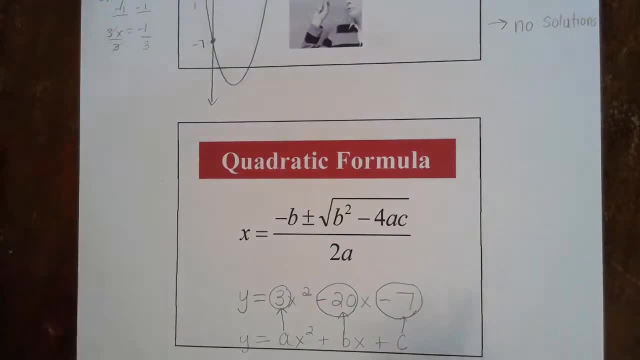 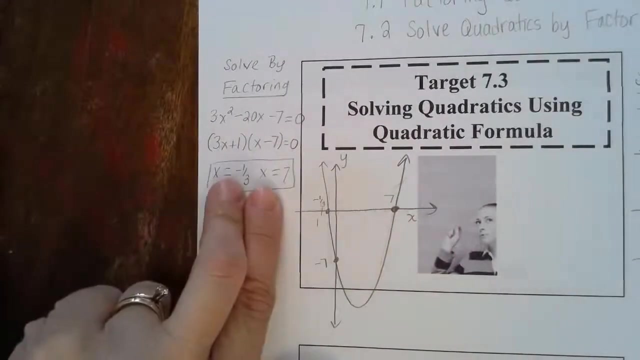 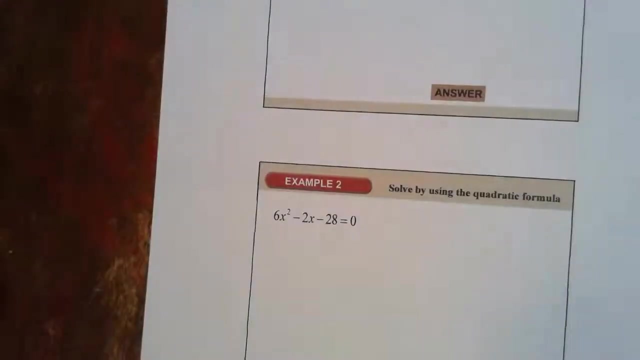 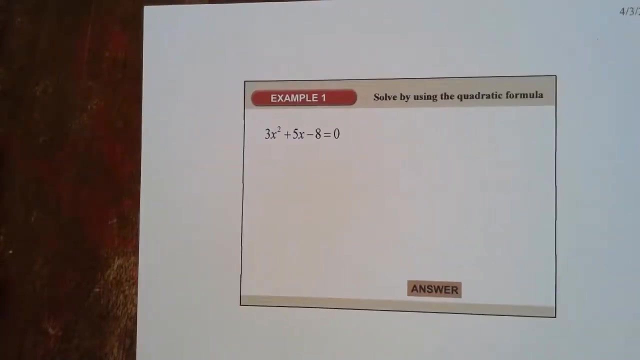 So I want to point that out before we actually do the equation. So I'm going to go ahead and do the two examples today. You have to be able to identify the parameters in order to use quadratic formula. And quadratic formula will get us to our solutions in another way instead of factoring. So let's go to, I think I only have two examples. Let's do the first one. It's a little bit different. I'm going to do this problem completely without the use of technology. And then I'm going to show you on decimals and on your graphing calculator. So in order to solve by using the quadratic formula, remember we're looking for where does it cross the x-axis. What values of x would make this a true statement if we plug in those values and evaluate? You first have to identify the parameters a and then b and then c. And I'm going to write quadratic formula off here to the left. Quadratic formula, 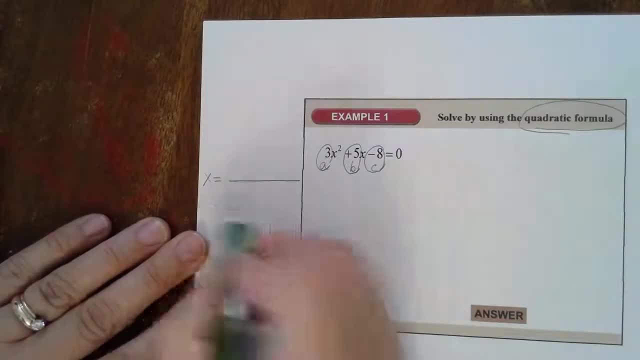 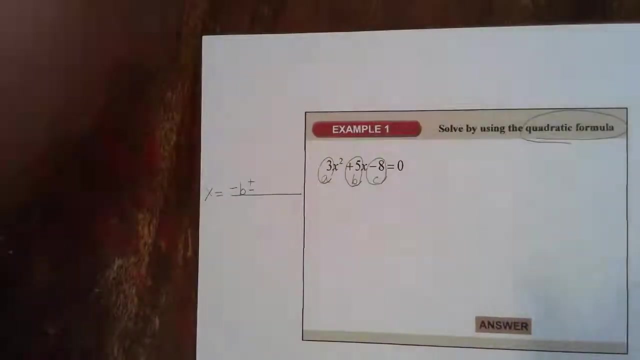 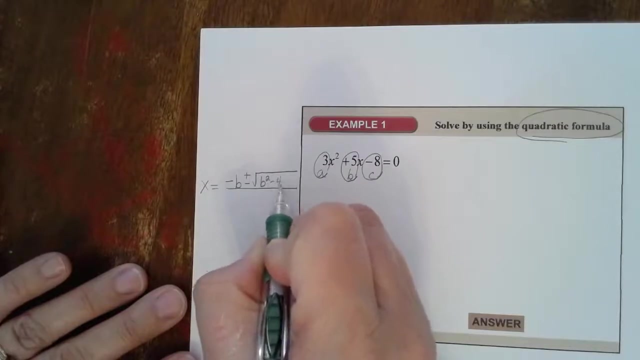 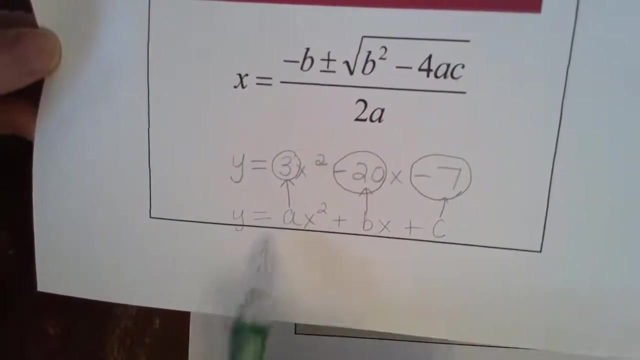 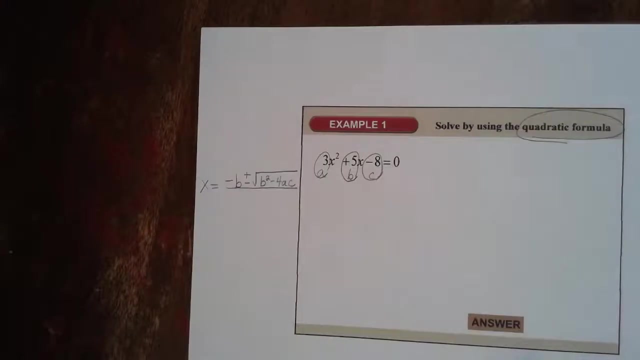 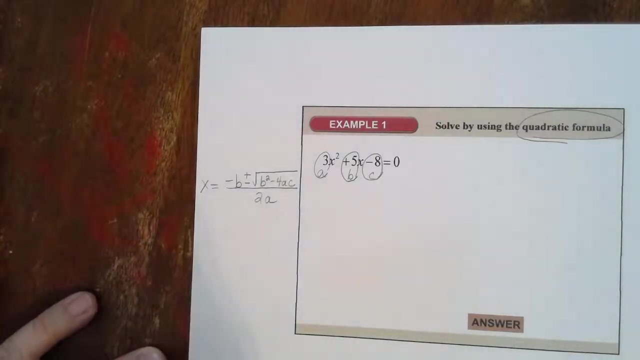 Algebra one is a quotient. It's a big fraction bar. And it's x equals because that's what you're solving for. It's the opposite of the b term. Plus or minus means that you'll have two answers potentially. Just like we had two answers over here. The plus and the minus takes into account the two possible answers. Then it's the square root of b squared minus four times a times c. The four product is always part of the formula. So we're going to use this formula. There's a reason for that. The reason is, it has to do with standard form of a quadratic equation. And if you were to solve that standard form for x by doing something called completing the square, you would get this number four. So the four is always part of the formula. So is this two a. The two is also part of the formula. So I'm going to use this formula and these parameters to solve. I'm going to write x is equal to b times c. And I'm going to write x is equal to b times c. So I'm going to use this formula. 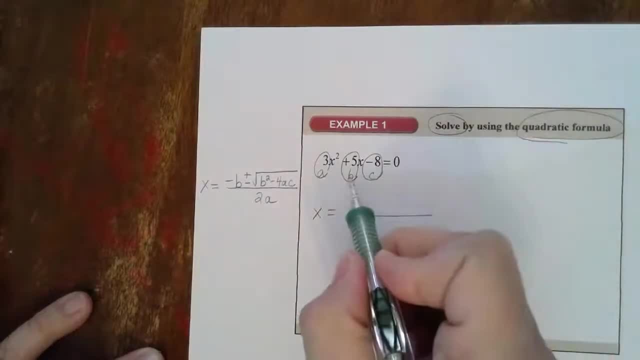 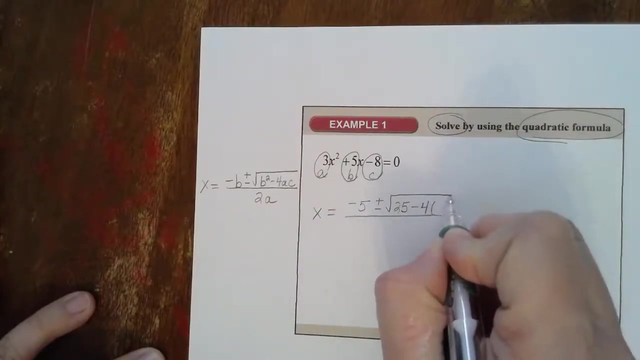 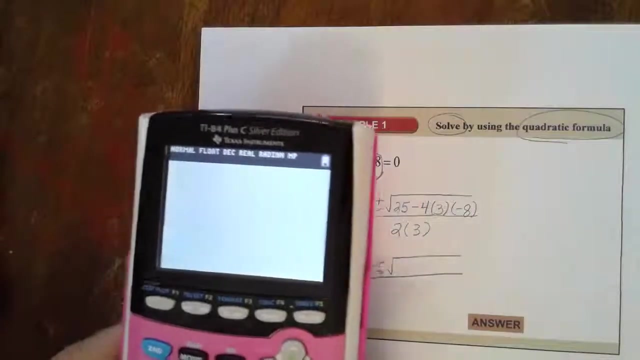 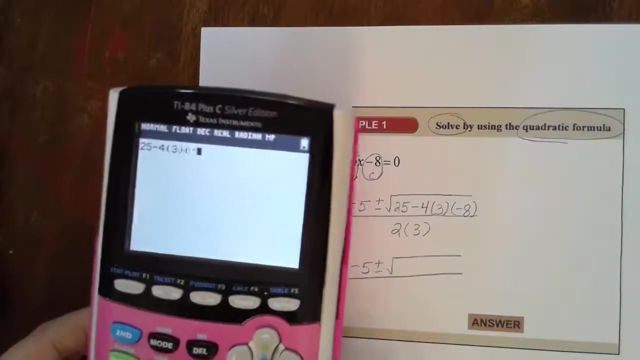 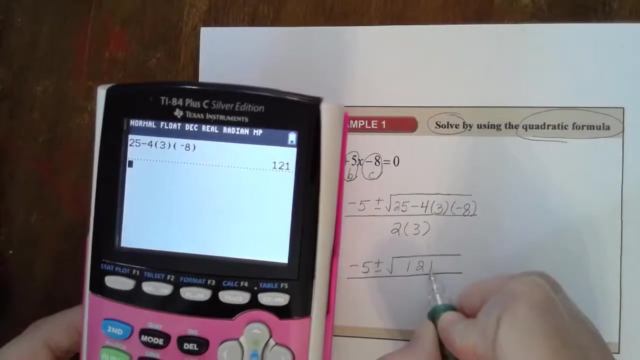 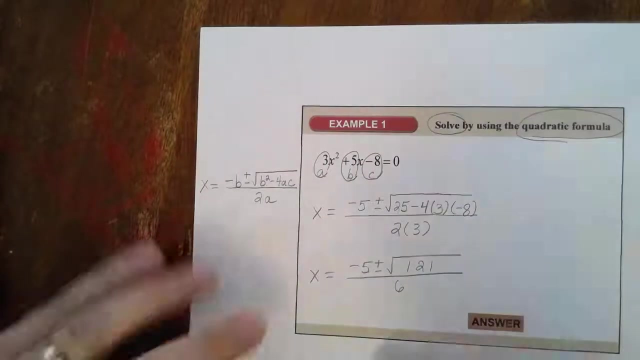 So I'm going to write x is equal to a big fraction bar. I'm going to do the opposite of the b term. The b term is five right now. So I'm going to do a negative five. I'm going to write plus or minus because then I'm going to separate those to do the two separate answers. Then the square root of. Now the thing is, the b is always squared. So no matter what you have for b, whether it's a positive or a negative, in this first term under the radical, that's always going to be a positive number. So the b is five. Five squared is twenty-five. Minus the number four times the product of four with a, which is the three, and then the c, which is negative eight. I'm going to divide all that by two times the a value, which is three. I'm going to simplify under the radical according to order of operations first. And when I simplify under the radical, I'm going to use my calculator to help me out a little bit. When I use my calculator, I'm going to do twenty-five minus four times three times negative eight. You could do that in your head if you wanted to. All of that will give me a hundred twenty-one. So underneath the radical, I have a hundred twenty-one divided by six. I probably, I said I wasn't going to use technology, but I just wanted to multiply that out just to reassure you. So I'm going 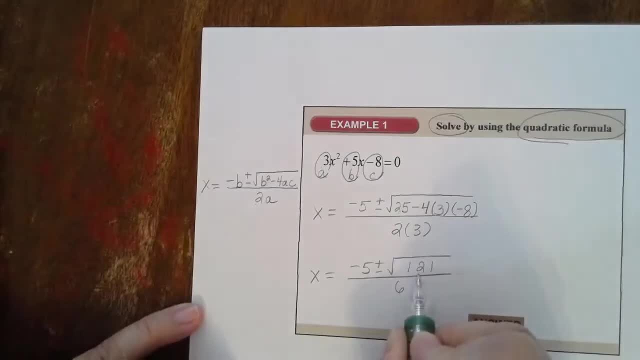 to do that. So I'm going to divide by six. So now I have this whole bunch of products and I'm going to divide by six. So I'm going to write this up in here. So I'm going to use my calculator and then out of three, I'm going to divide by six. And then out of five, I'm going to divide that by six. So this is the total. This is what works. One will be the total of the product and the other will be the total of the product. So I'll divide by six, not Negative 5 minus 11 divided by 6. Simplifying a little more, let's do negative 5 plus 11, which is positive 6, divided by 6. So one of the answers is 1. 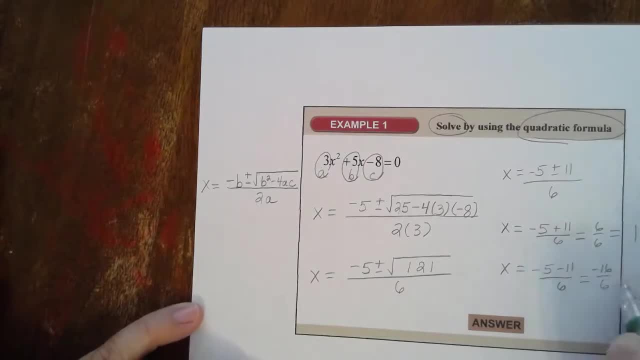 Then this would be negative 5 minus 11, negative 16 all over 6. I'm going to reduce that to negative 8 thirds because 2 goes into 16. 8 times 2 goes into 6, 3 times. So my two answers are 1 and negative 8 thirds. 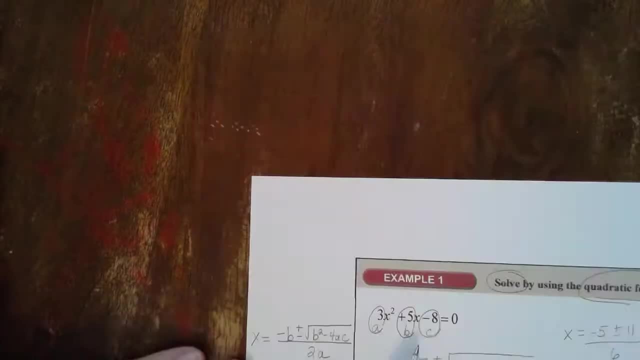 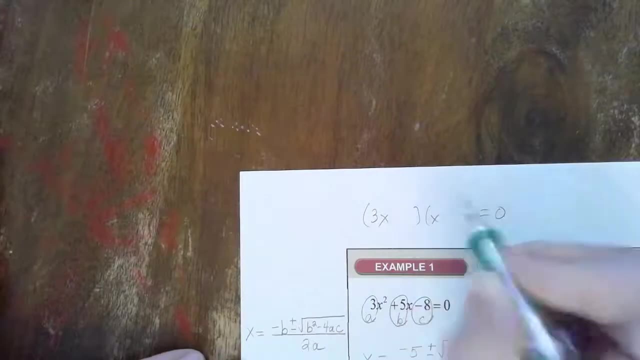 Now we could have factored that. We could have taken this and we could have gone, I'm going to factor up here, equals 0, 3x and x will give me 3x squared, negative 8. I know is probably 4 times 2, but I already know my two answers down here. So I'm going to write, I know 8 is 8 and 1. 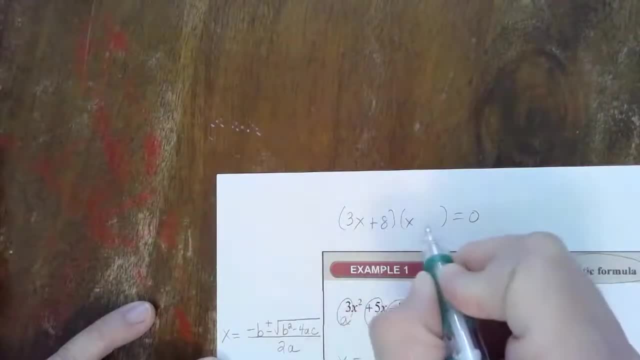 But I'm going to write a positive 8 here and a negative 1 here. And if I want to get 5 in the middle, that's going to be 8x minus 3x gives me my 5x. So my two answers are positive 1 and when I subtract 8 from both sides by setting it equal to 0, notice I get the same answers by factoring. 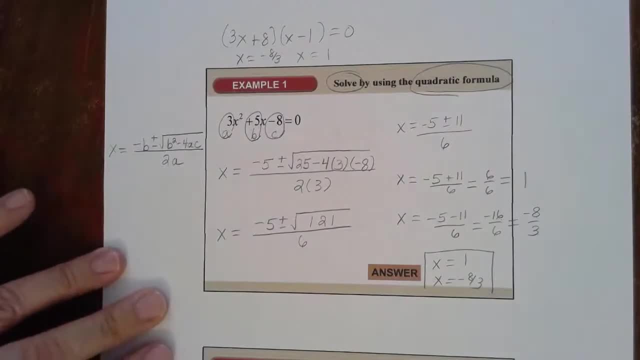 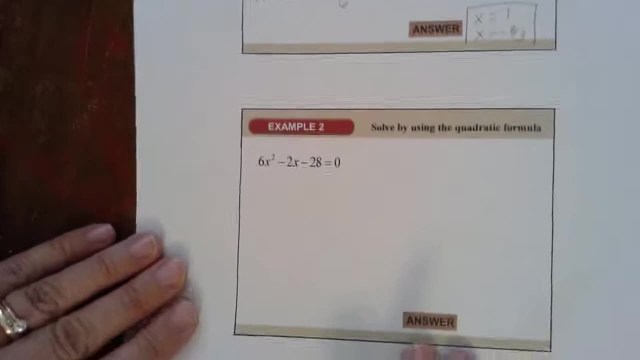 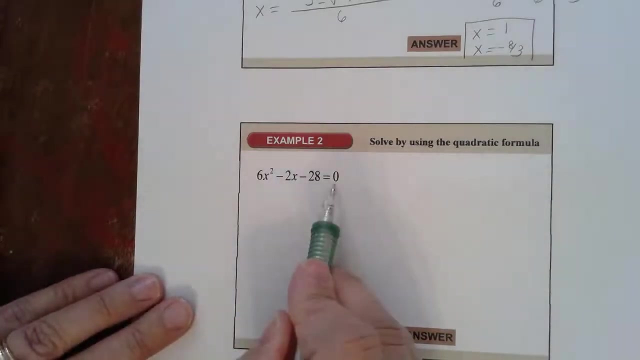 The thing about quadratic formula though, it can solve any quadratic equation. Okay, so now this next one I'm going to do entirely on my computer and in decimals, I mean, and also on a graphing calculator. I still have to identify the parameters. It has to be in standard form. So if 28 were over on the other side, I'd have to move it. 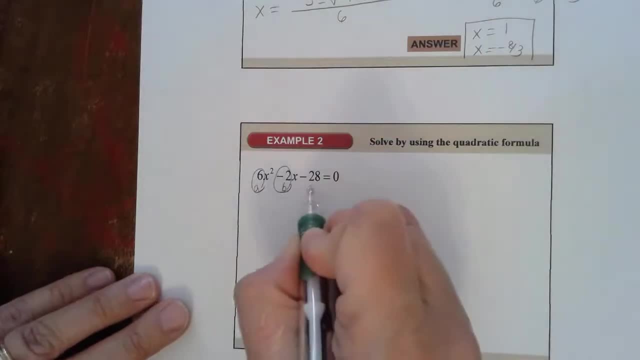 So a is 6, b is negative 2, and c is negative 28. 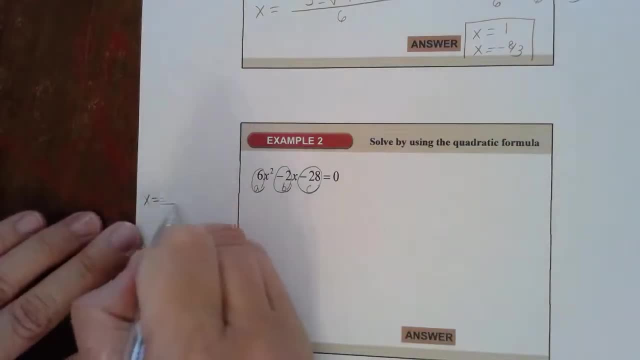 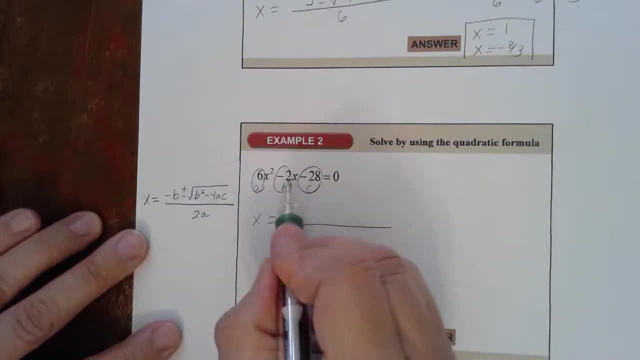 My quadratic formula, I'm going to write out quickly over here so we can reference it every time. And I'm going to go right into plugging everything in. So I'm going to do the opposite of the b term. Right now I have a negative 2, so I'm going to put a positive 2 plus or minus square root. Then I have to square the b term. b is negative 2, but negative 2 times negative 2 is positive 4. This will always end up with a positive value. 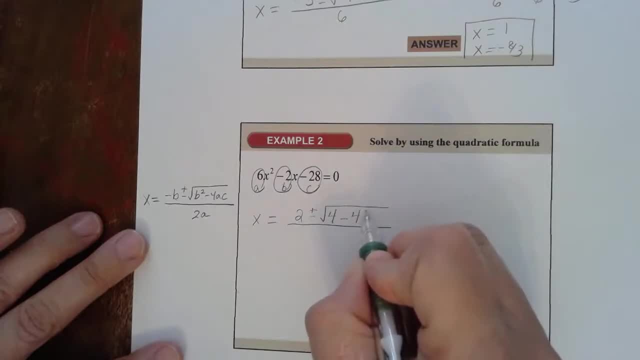 So 4 is because it's negative 2 times negative 2, then minus another 4. 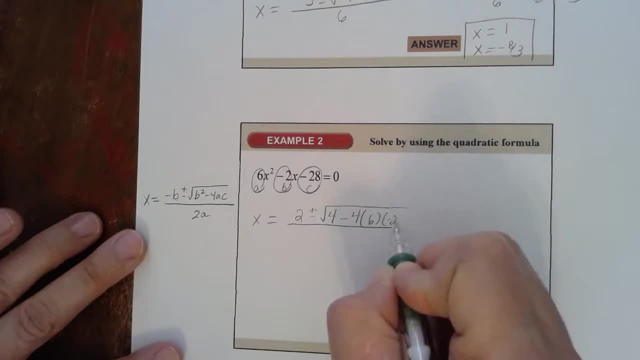 And then a is 6, and c is negative 28. All over 2 times 6. 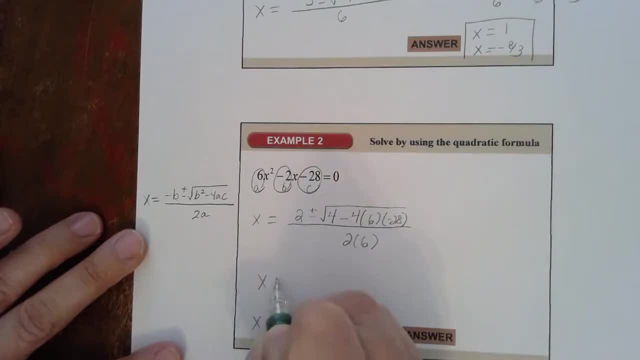 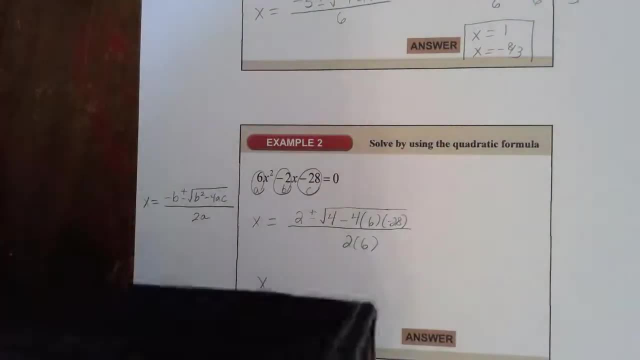 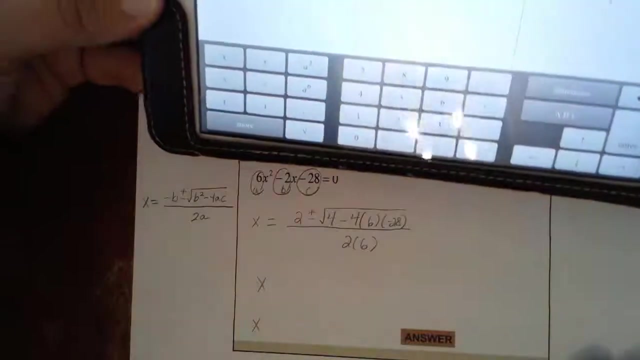 Now, what I'm going to do here is I am going to use decimals in order to solve this quadratic equation. I'm going to use it on my iPad. And so, let's see how this will work. I want to show what I'm plugging in. So I'm going to kind of move this. I'm going to move this guy over here. 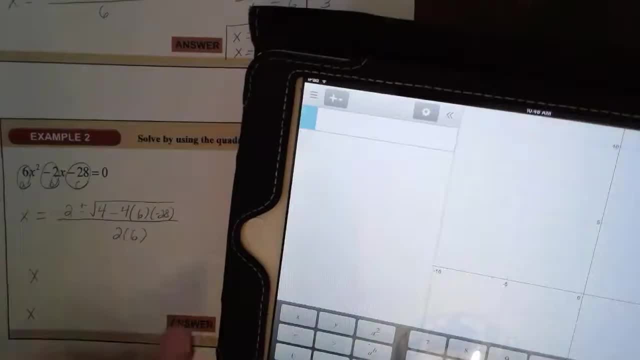 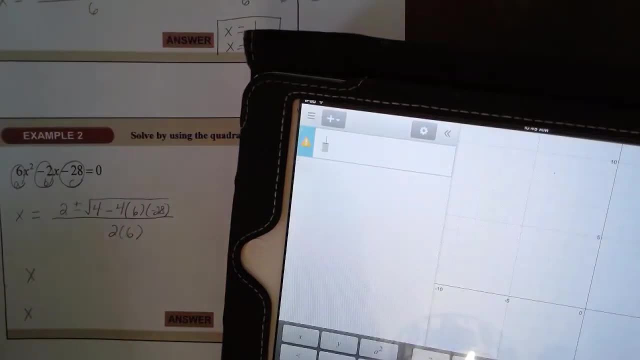 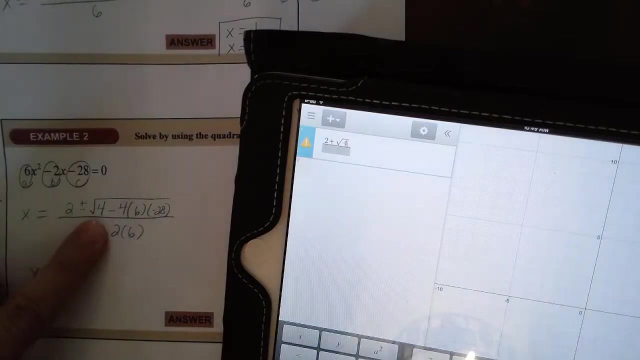 And hopefully you can see my decimals work right here. So I'm in decimals, and I'm going to type this guy in just as I see it, but I have to do the plus and minus separately. I'm going to hit a division bar right away. Then 2. Then I'm going to do my plus. Then I have my square root key right here. And then I have 4 minus 4. And then in parentheses times 2. 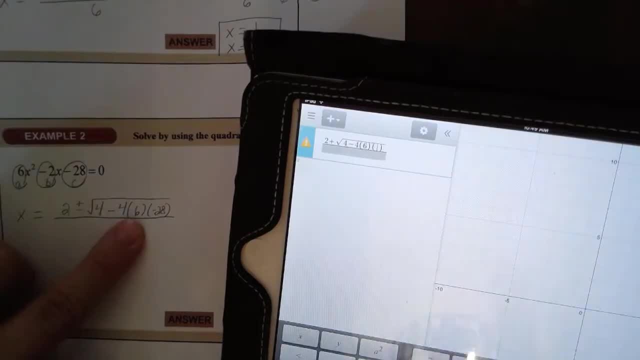 And then in parentheses, in decimals, the negative and minus are the same. Negative 28. 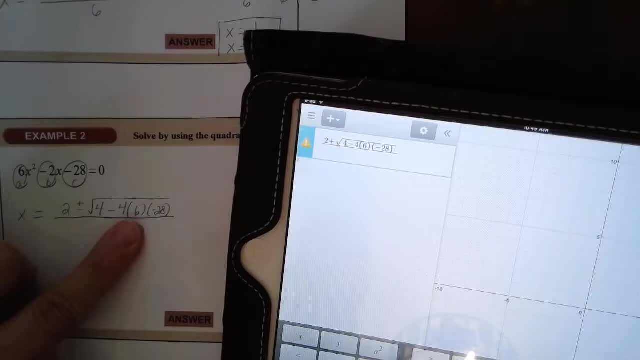 Then I'm going to arrow down, I think. There we go. And my denominator is 2 times 6. So I'm just going to put the number 12. 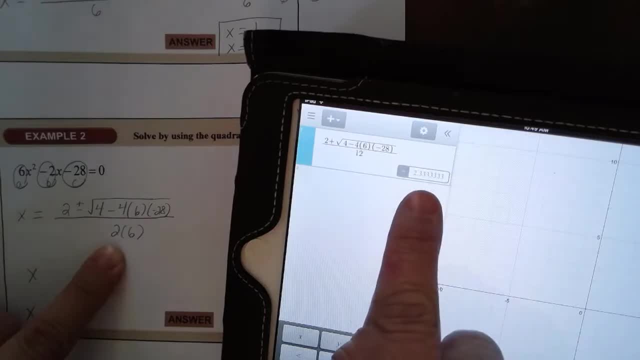 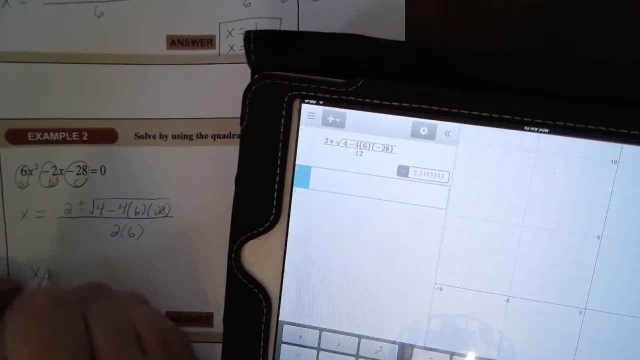 Then notice I get one of my answers, 2.3 repeating. So I'm going to write one of my answers is approximately 2.3. 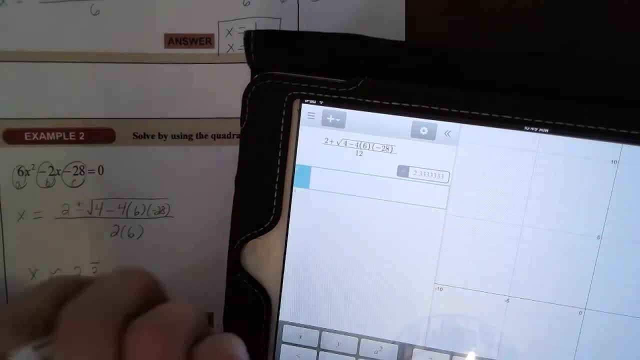 Or you could write that's 8 thirds, I believe. 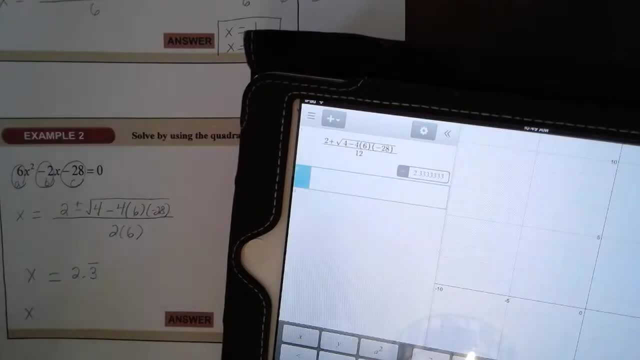 Believe it or not, we got a similar answer. Then to get the other answer, I'm just going to go back up into decimals. And I'm going to change that plus to a minus. And get my other answer right away, negative 2. 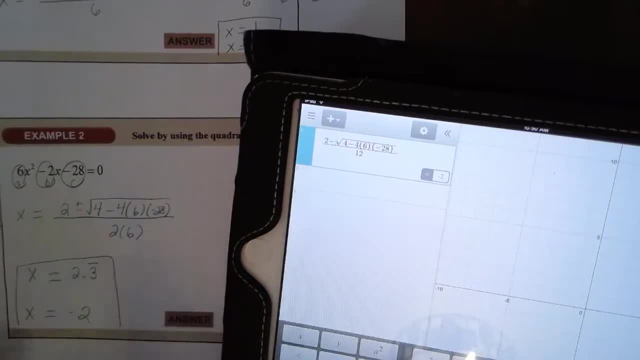 So there are my two answers. In another day in quadratic formula, we'll get some irrational numbers. Both of these are rational, 2.3 repeating and negative 2. 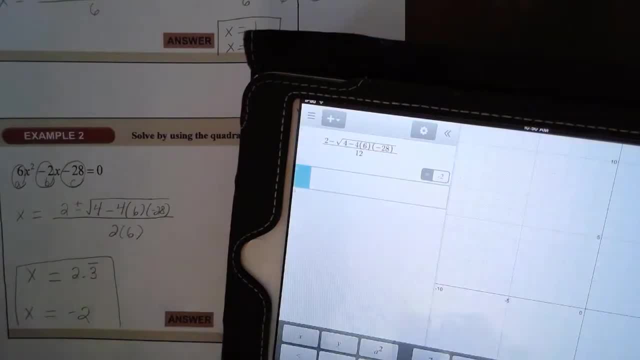 If I wanted to, I could graph this, too. I'm going to type this in as y equals 6x squared, then minus 2x, then minus 28. Now, that's a really big y-intercept, but hopefully you can see, and I'm not sure how to minimize this, but that's okay.